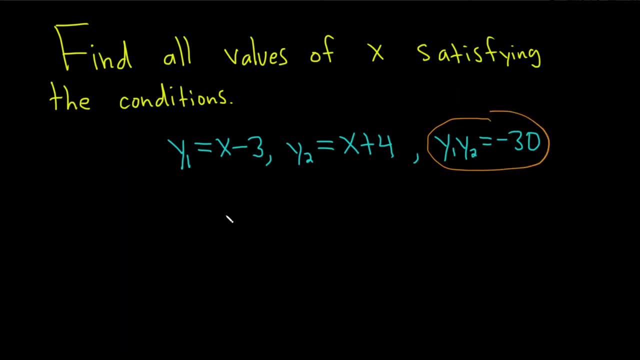 start maybe by using this and then just plugging these into this equation. So solution SOL means solution. So y1, y2 equals negative 30. You have write that down. Okay, let's replace y1 with what it is: It's x minus 3.. So x minus 3, and then y2 is x plus 4.. 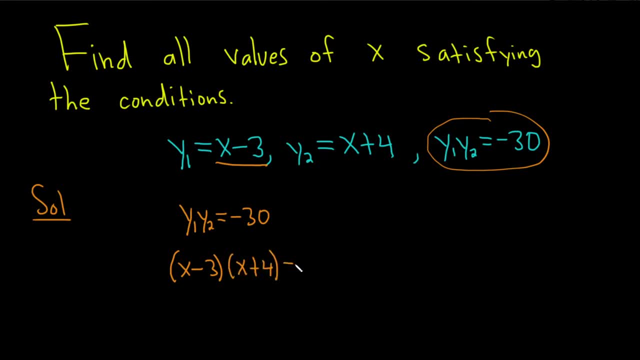 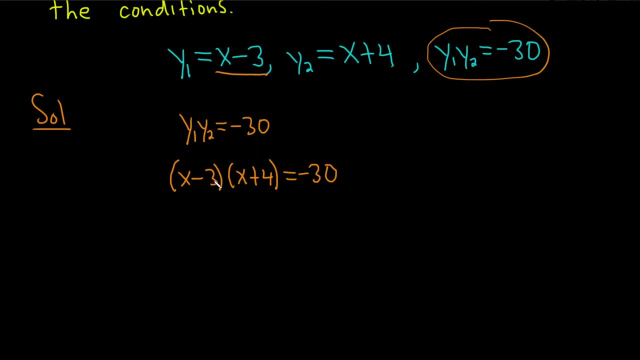 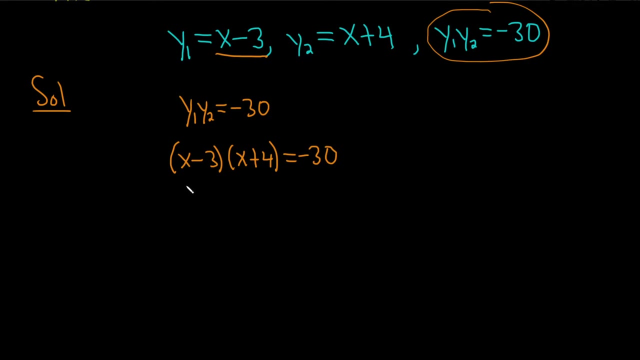 x plus 4, and this is equal to negative 30. So now we should multiply this out. You see, this is going to be a quadratic equation, and so whenever you have a quadratic equation, typically you want to try to set it equal to zero to try to solve it. So you're going to want to set it equal to zero. 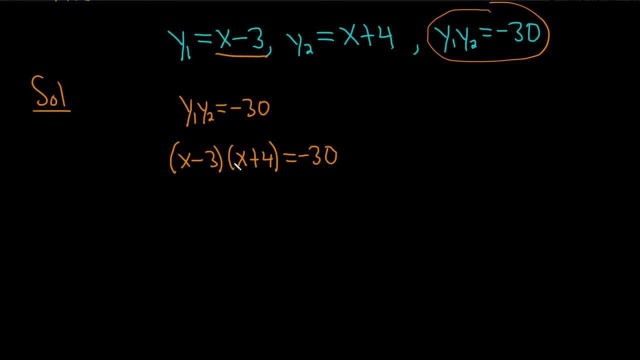 so let's distribute here. We'll take the x and multiply it by both of these. So x times x is x. squared x times 4 is 4x. Then negative 3 times x, is just negative 3 times x, And then negative 3. 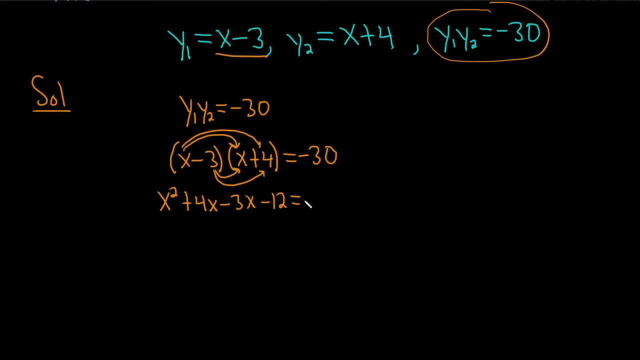 times 4 is negative 12. And that's equal to negative 30.. Let's combine like terms here. So this is x squared 4x, is x squared 4x is minus 3x, It's just 1x, So you can just put an x, Then minus 12. And that's equal to. 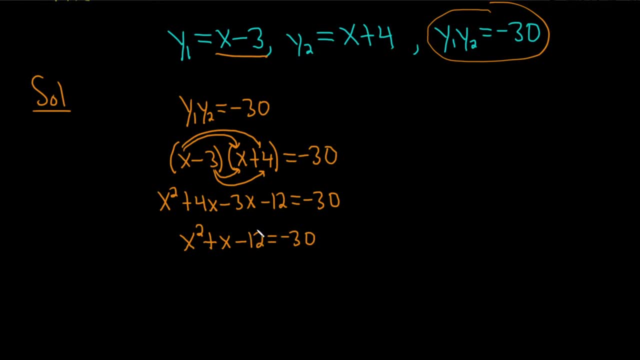 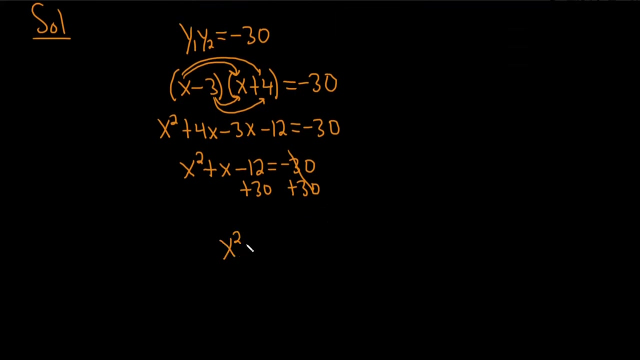 negative 30.. And again, it's a quadratic equation, So we definitely want to set it equal to zero. So we'll add 30 now to both sides. So plus 30 plus 30. These cancel, So we get x squared. plus x Looks like plus 18.. 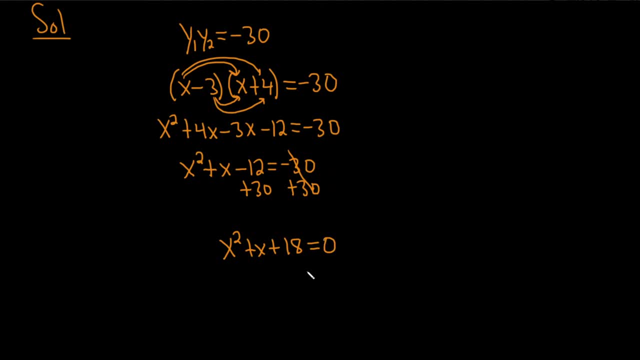 And that's equal to zero. Hmm, Does this factor? I'm thinking hard here. So what numbers multiply to 18 and add to 1? I don't really know. Like 3 and 6 give us 18.. 2 and 9 give us 18.. 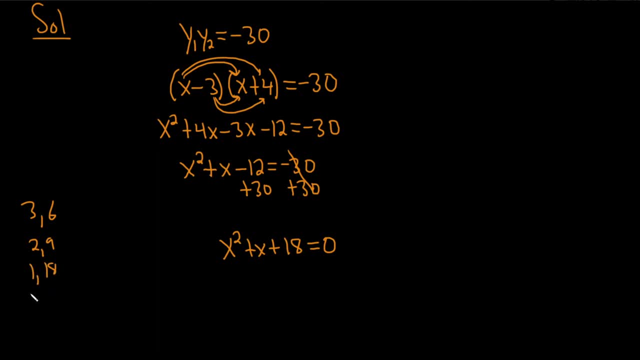 1 and 18 give us 18.. I can't really think of anything else, right? I mean, the factors of 18 are 2, 3, etc. So it's 2 times 9.. So it's 2 times 3 squared. 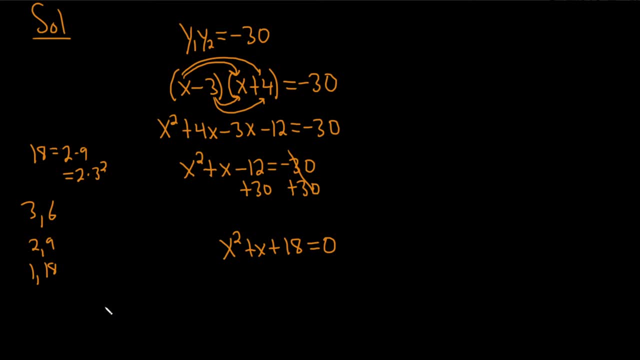 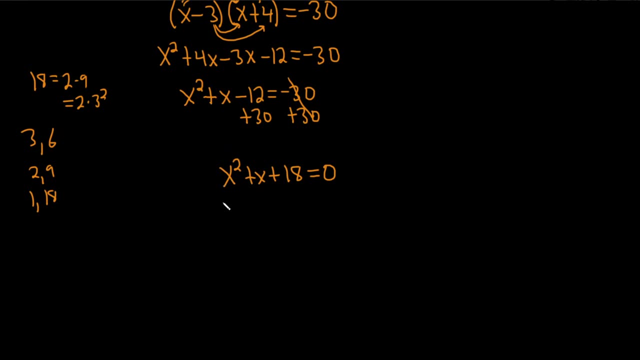 So yeah, I think that's pretty good, pretty much it. So let's go ahead and try to use the quadratic formula now. So, to use the quadratic formula, we have to identify a, b and c, So we can think of this as ax squared plus bx plus c. 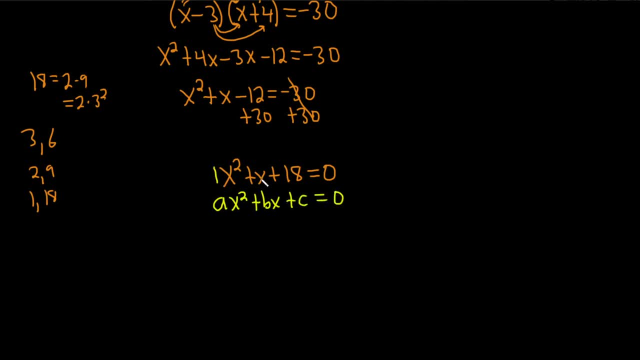 equals 0. So using matching- we know there's ones here- So a is 1,, b is 1, and c is 18.. So the quadratic formula says that x is equal to negative b plus or minus the square root of. 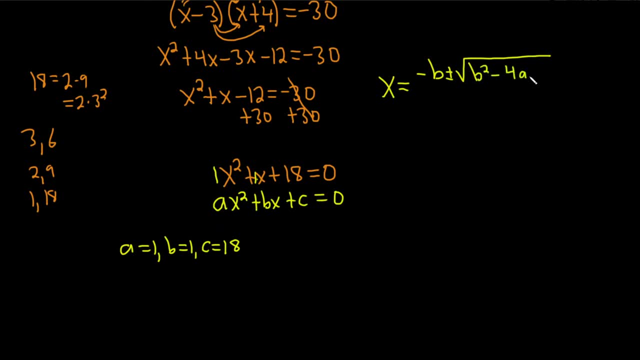 b squared minus 4ac, And it's all over 2a. So x is equal to, so b is 1, so this will be negative: 1 plus or minus the square root of 1 squared, that's your b. 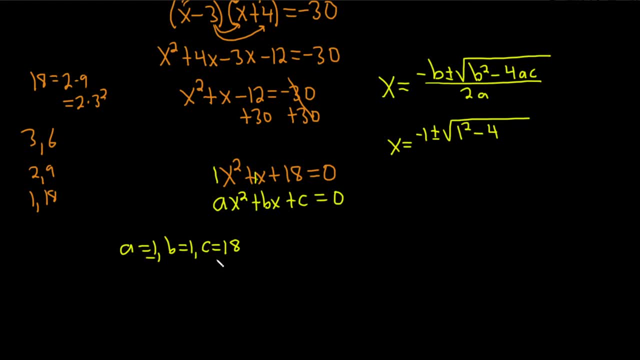 b squared minus 4ac And it's all over 2a. So x is equal to, so b is 1, so this will be minus four ac. so one times eighteen big numbers. huh, pretty tough problem. i have not done this before. uh, making this video i usually don't usually just do them on the spot. and two times. 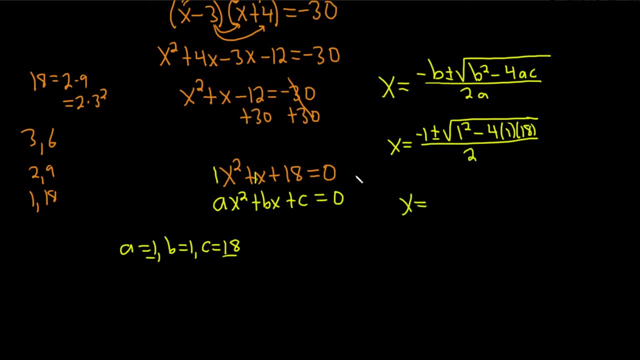 one is two. pretty tough, i thought. i thought this would factor. i was hoping it would be nice, but it's too hard to factor with our minds, so good way to go: negative one plus or minus. let's see here: oh, four times eighteen. i believe that is sixty four. i'm just triple checking. no, it's seventy. 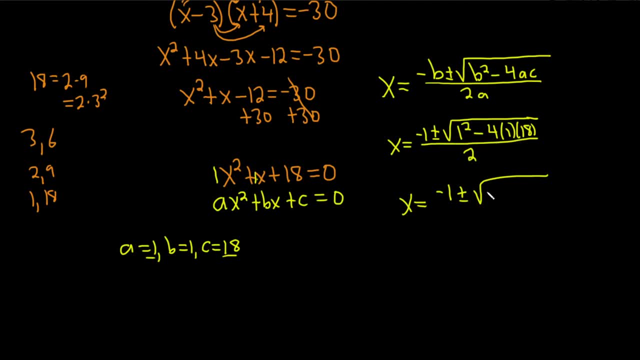 two. brain brain, uh fart. so one minus seventy two. brain failure over two. so x equals negative one plus or minus. uh, the square root of negative seventy one over two and the square root of seventy one is not something we know. really, it's not something nice, so we're just going to get an i. 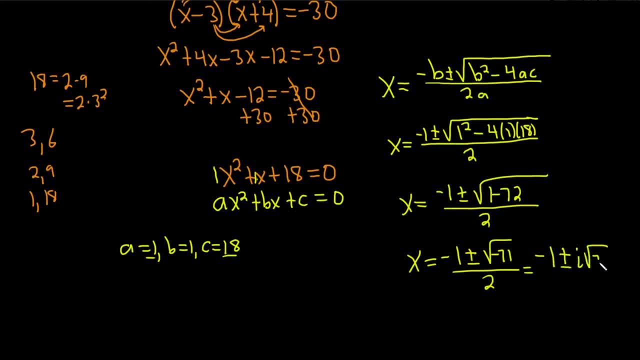 now because of the negative. so this is i square root of seventy one over two, and that would be the final answer. i hope this video has been helpful. good luck.